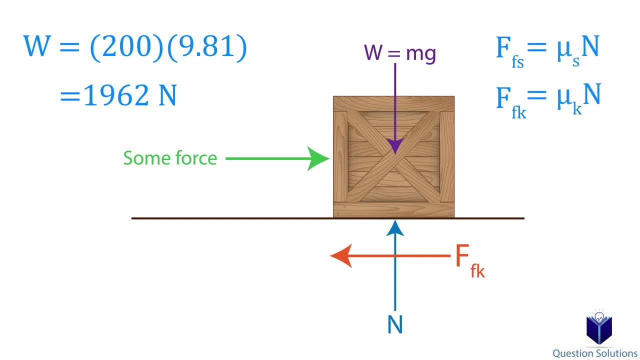 Frictional force is calculated by multiplying the coefficient of friction by the normal force. So in most cases you would find the normal force first and then multiply it by the coefficient of friction to find the frictional force. Now that we got that covered, let's move on to some examples. 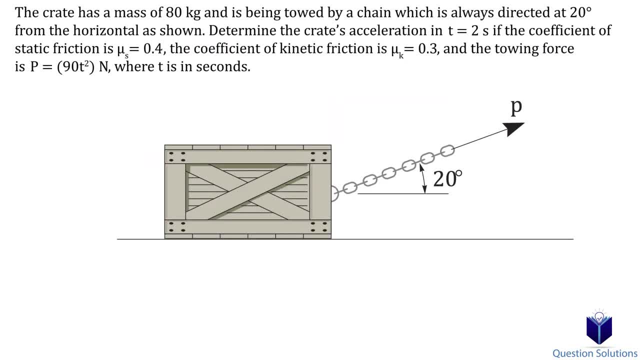 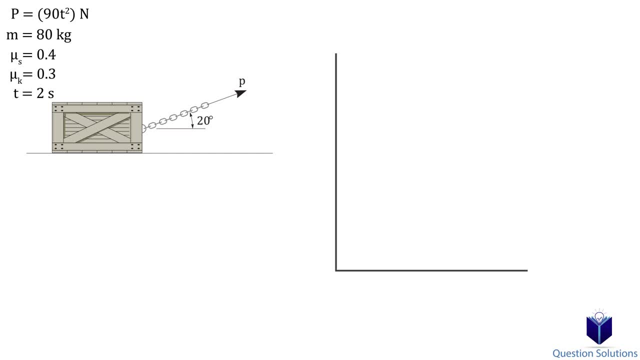 In this problem we need to determine the crate's acceleration in 2 seconds. So the force given to us in the question is with respect to time. In other words, as time goes by, the force applied to the chain gets bigger. So let's think about this problem. The force must. 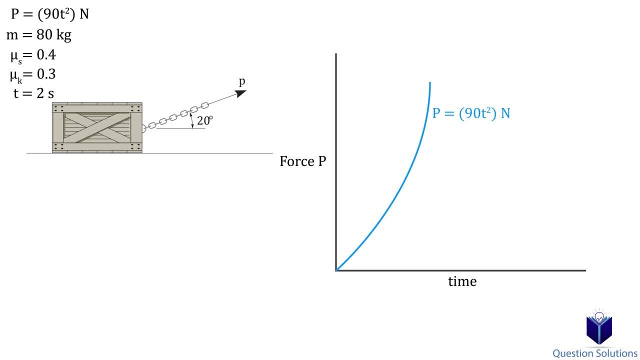 increase over time until the crate begins to move. Another way of thinking about it is that the force must overcome the friction created between the crate and the floor. Until it does, the crate stays still. The first step is to actually make sure that at 2 seconds the crate can move. So if 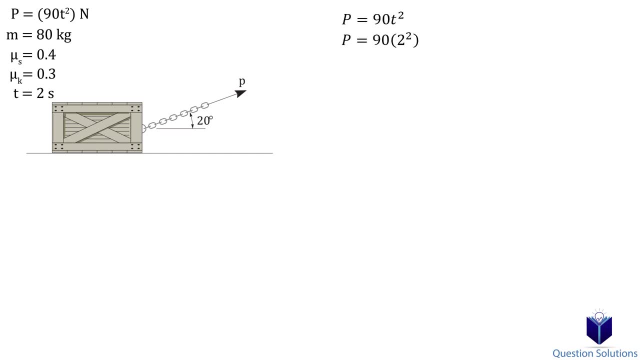 we plug in 2 seconds into the equation representing force, we get 360 newtons. Now let's draw a free body diagram labeling the force applied to the chain. The force applied to the chain gets bigger. So if we take the force applied to the chain, we get the force applied to the crate. We have force. 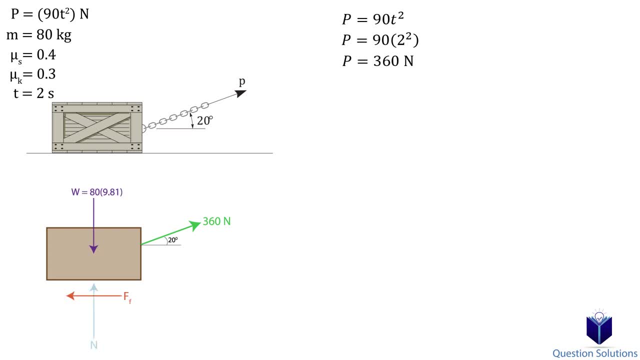 p: the weight, the frictional force and the normal force. Friction always points opposite to the direction the crate would move. Since we're trying to see if the crate will move at 2 seconds, we need to see if the force applied can overcome the frictional force. So we will write an equation. 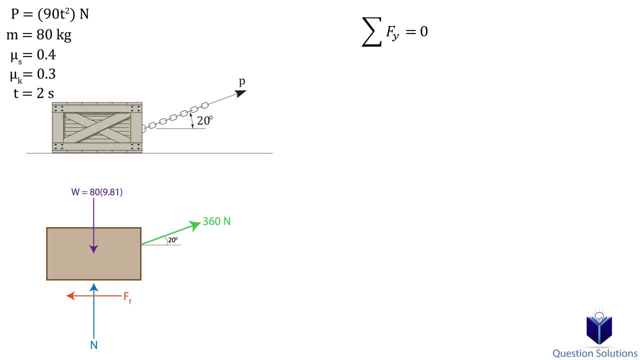 of equilibrium. That simply means all the forces added together will equal 0.. We write an equation of equilibrium when the object is not moving. When we do that, we consider the force applied to the chain as static friction, not kinetic friction. Let's write the first equation for forces in the 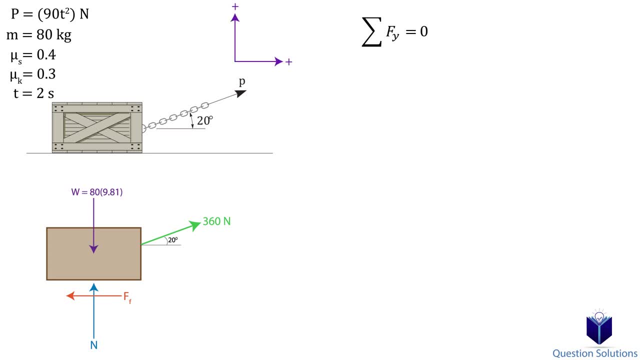 vertical direction. We will assume forces upwards to be positive. So we have the normal force, the y-component of the p-force and the weight which is downwards, and all of that added together is equal to 0.. Let's solve for the normal force. The next step is to write another equation of. 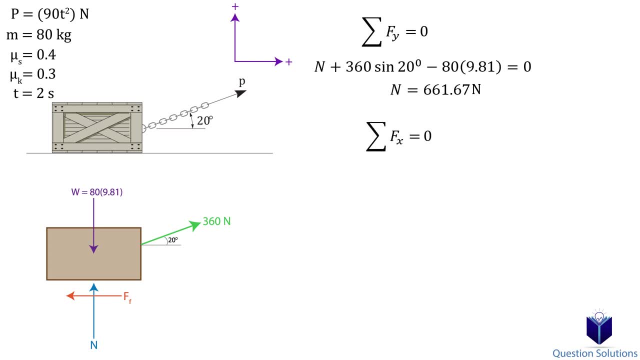 equilibrium for the horizontal forces. So we have the x-component of force p and the frictional force. Let's solve for the frictional force. This value we found represents the frictional force required to keep the box from moving at 2 seconds. Another way of thinking is that this is the frictional 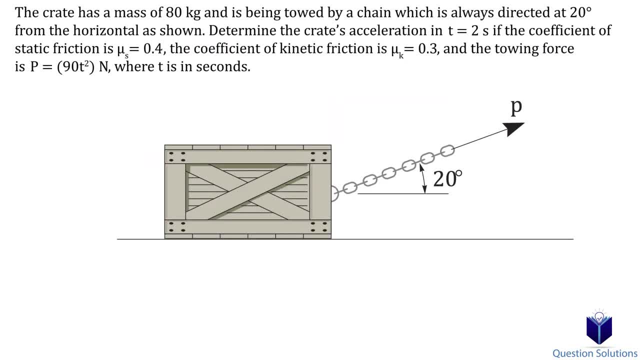 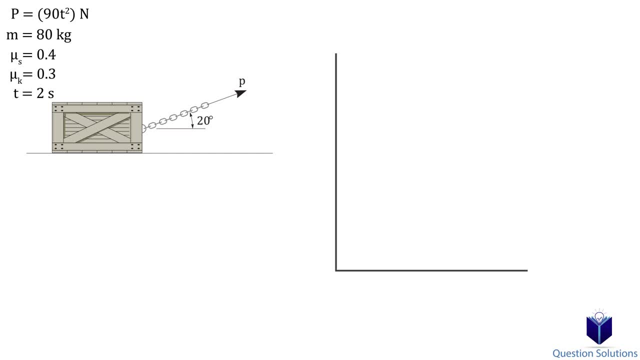 In this problem we need to determine the crate's acceleration in 2 seconds. So the force given to us in the question is with respect to time. In other words, as time goes by, the force applied to the chain gets bigger. So let's think about this problem. The force must. 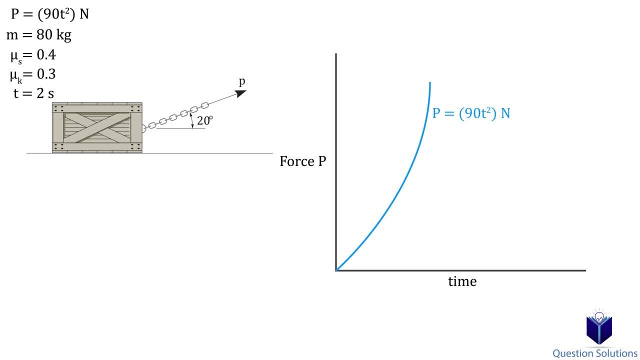 increase over time until the crate begins to move. Another way of thinking about it is that the force must overcome the friction created between the crate and the floor. Until it does, the crate stays still. The first step is to actually make sure that at 2 seconds the crate can move. So if 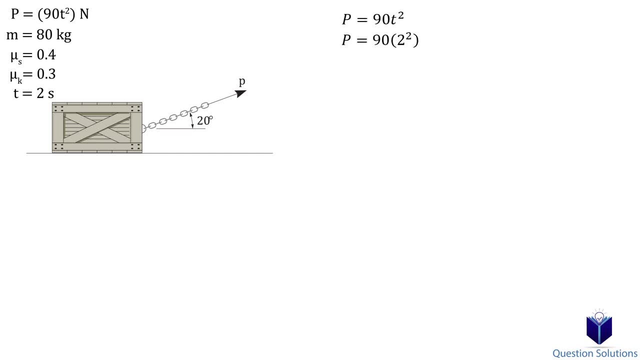 we plug in 2 seconds into the equation representing force, we get 360 newtons. Now let's draw a free body diagram labeling the force applied to the chain. The force applied to the chain gets bigger. So let's draw a free body diagram labeling the force applied to the chain. The force applied to the 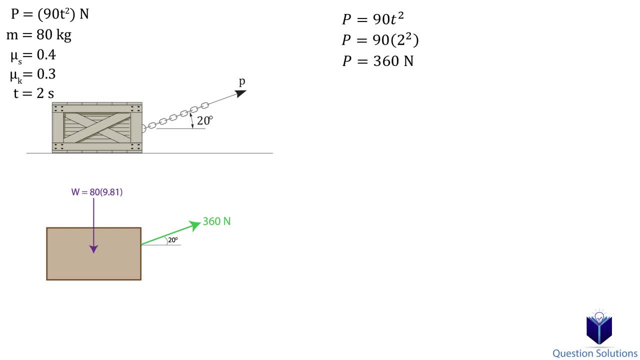 chain gets bigger. So let's draw a free body diagram labeling the force applied to the chain gets bigger. We have force P, the weight, the frictional force and the normal force. Friction always points opposite to the direction the crate would move. Since we're trying to see if the crate will move, 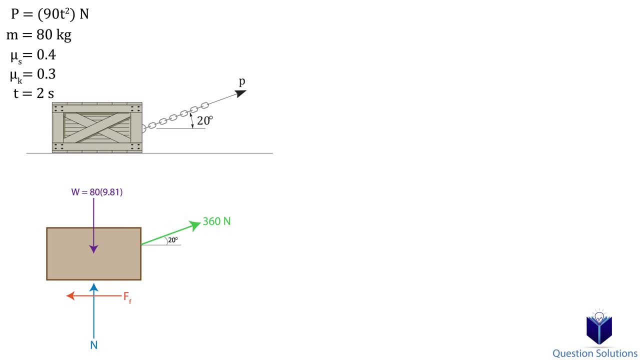 at 2 seconds. we need to see if the force applied can overcome the frictional force. So we will write an equation of equilibrium That simply means all the forces added together will equal zero. We write an equation of equilibrium when the object is not moving. When we do that, 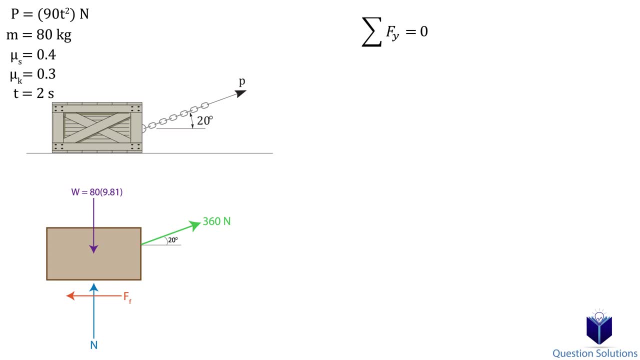 we consider the force applied to the chain as the force applied to the chain. So we can see that the force applied to the chain is the force applied to the chain. We consider the static friction, not kinetic friction. Let's write the first equation for forces in the vertical direction. 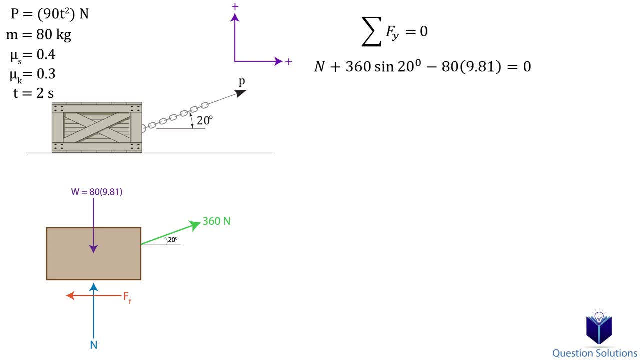 We will assume forces upwards to be positive. So we have the normal force, the y component of the P force and the weight which is downwards, and all of that added together is equal to zero. Let's solve for the normal force. The next step is to write another equation of equilibrium. 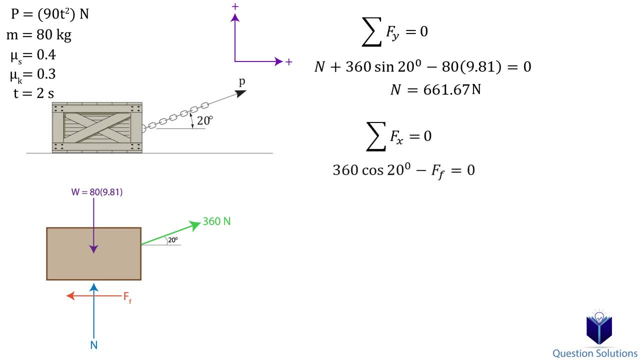 for the horizontal forces. So we have the x component of force P and the frictional force. Let's solve for the frictional force. This value we found represents the frictional force required to keep the box from moving at 2 seconds. Another way of thinking is that this: 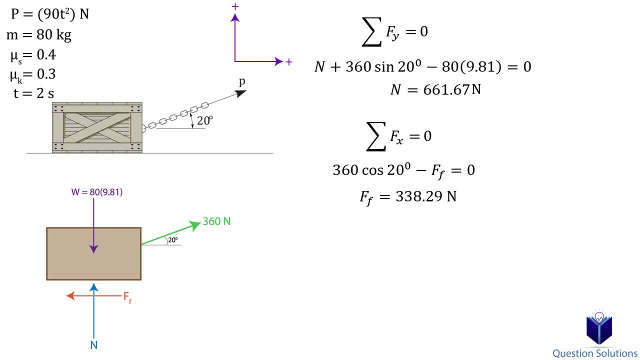 is the frictional force required to counteract the pulling force at the chain. Now let's find the maximum friction that can occur with the coefficient of static friction given to us. That's simply the normal force multiplied by the coefficient of static friction. So from our calculations we see that the maximum frictional force that can occur 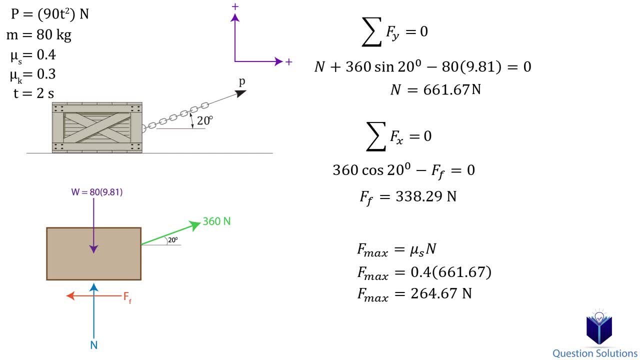 is 264 newtons, while the required frictional force to keep the box from moving at 2 seconds is 338 newtons. Since the maximum frictional force is smaller, that means the box will be moving at 2 seconds. Now that we know this, we can move on to the next step, which is to figure out. 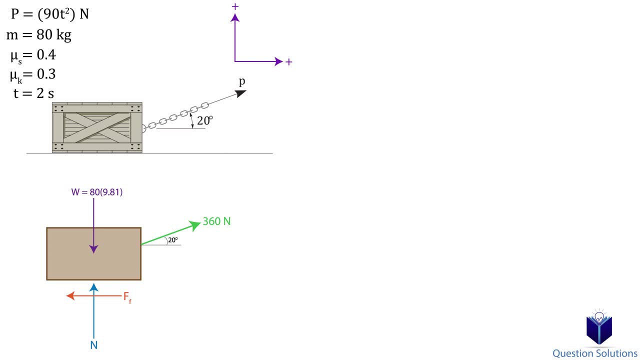 the crate's acceleration in 2 seconds. For that we will write up equations of motion. That's when we write: F equals ma. So again we will write an equation for vertical movement. We have the normal force, the weight, the y component of force, p, and all of that added together is equal to the. 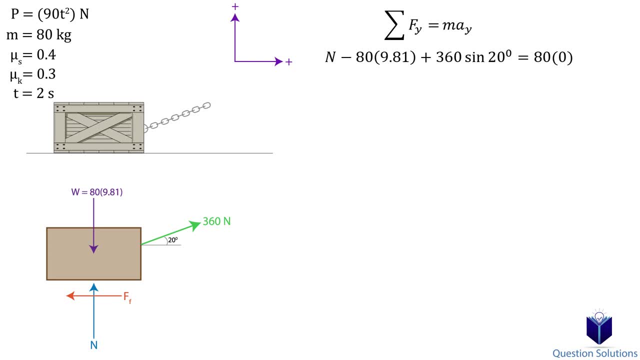 mass multiplied by acceleration. But remember the crate is only moving to the side, not upwards, so our acceleration upwards is zero. Let's solve for the normal force. Now let's write another equation of motion for horizontal forces. This time we have the x component of force p. 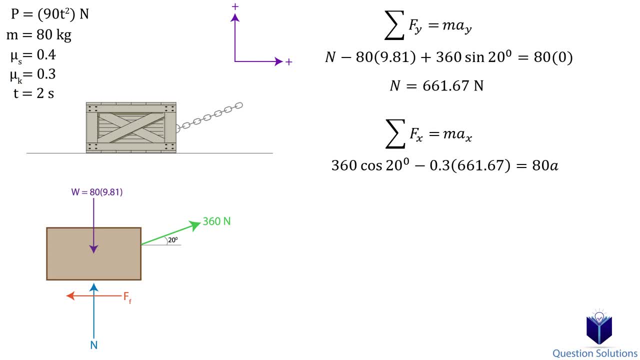 the frictional force with the coefficient of kinetic friction multiplied by the normal force, and all of that added together is equal to the mass times acceleration. Let's solve for the acceleration, And that's our answer. Now you might think: well, why didn't we just solve for this? 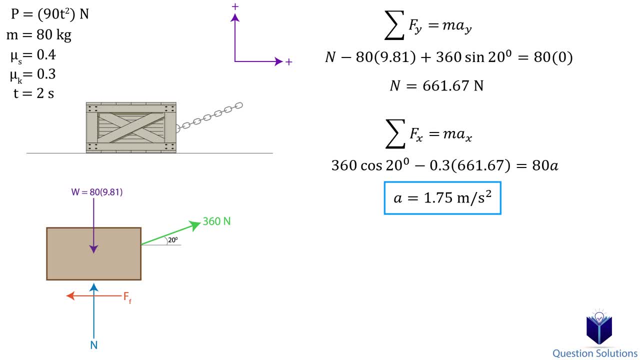 Why did we go through a bunch of steps trying to show that the crate will move at 2 seconds? That's because if our coefficient of static friction was higher- meaning the frictional force was lower than the maximum frictional force, then the crate would not move in 2 seconds. But 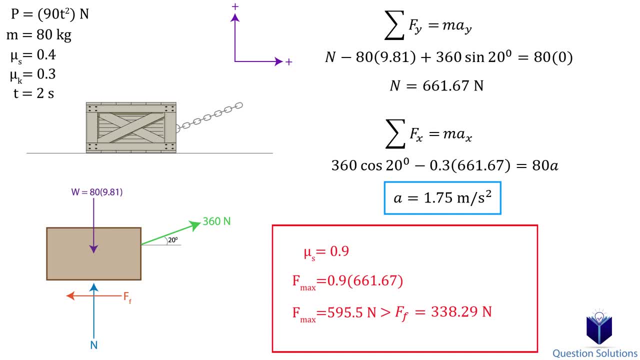 you can still write equations of motion and find an acceleration, because you're using the coefficient of kinetic friction, The only difference being it's not a practically valid answer. The crate will not be moving, so while you can get an acceleration, it won't make any sense. 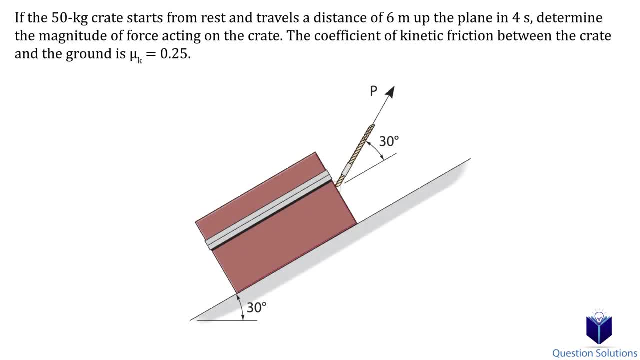 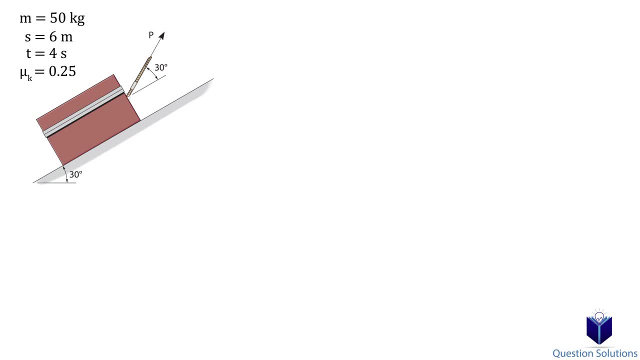 Let's look at another problem In this question. we need to figure out the force applied at the rope for the crate to move a distance of 6 meters in 4 seconds. We can start off by drawing a free body diagram. So we have force p, the weight which is always straight down the normal force. 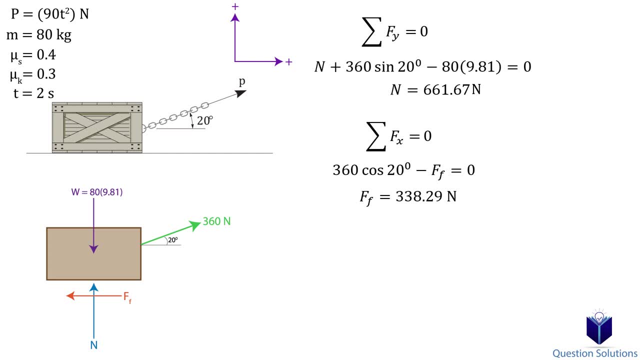 force required to counteract the pulling force at the chain. Now let's find the maximum friction that can occur with the coefficient of static friction given to us. That's simply the normal force multiplied by the coefficient of static friction. So from our calculations we see that 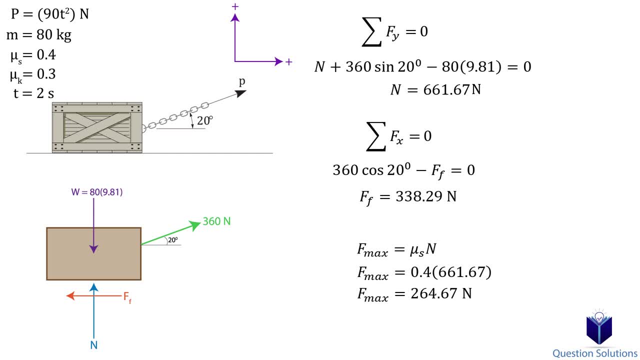 the maximum frictional force that can occur with the coefficient of static friction given to us is 264 newtons, while the required frictional force to keep the box from moving at 2 seconds is 338 newtons. Since the maximum frictional force is smaller, that means the box will be moving at 2. 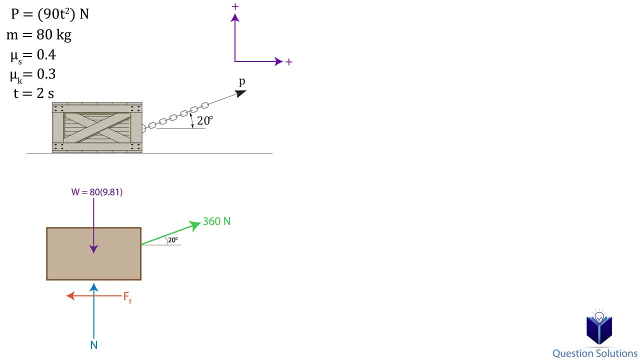 seconds. Now that we know this, we can move on to the next step, which is to figure out the crate's acceleration in 2 seconds. For that we will write up equations of motion. That's when we write f equals ma. So again we will write an equation for vertical movement. We have the normal force. 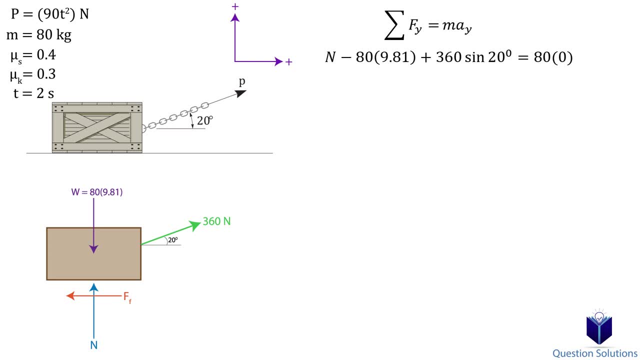 the weight, the y component of force p and all of that added together is equal to the mass multiplied by acceleration. But remember, the crate is only moving to the side, not upwards, So our acceleration upwards is zero. Let's solve for the normal force. Now let's write another. 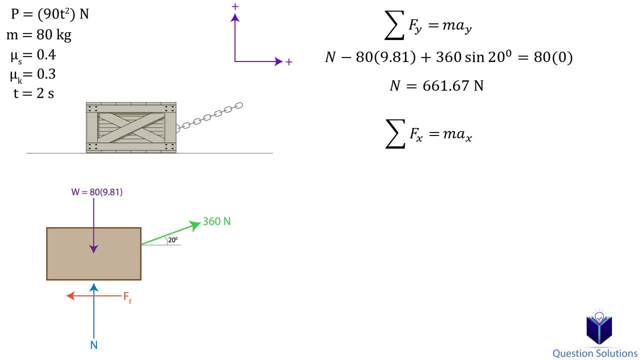 equation of motion for horizontal forces. This time we have the x component of force p, the frictional force with the coefficient of kinetic friction multiplied by the normal force, and all of that added together is equal to the mass times acceleration. Let's solve for the acceleration, And that's our answer. Now you might think: well, why didn't we? 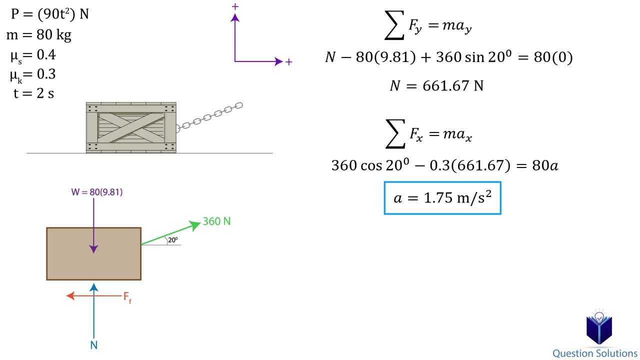 just solve for this. Why did we go through a bunch of steps trying to show that the crate will move at 2 seconds? That's because if our coefficient of static friction was higher- meaning the frictional force was lower than the maximum frictional force, then the crate would not move in 2 seconds. But 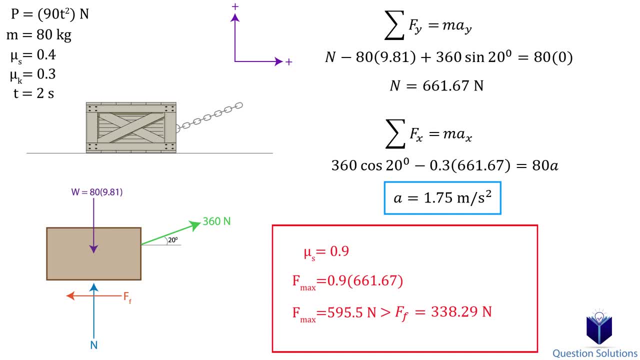 you can still write equations of motion and find an acceleration, because you're using the coefficient of kinetic friction, The only difference being it's not a practically valid answer. The crate will not be moving, so while you can get an acceleration, it won't make any sense. 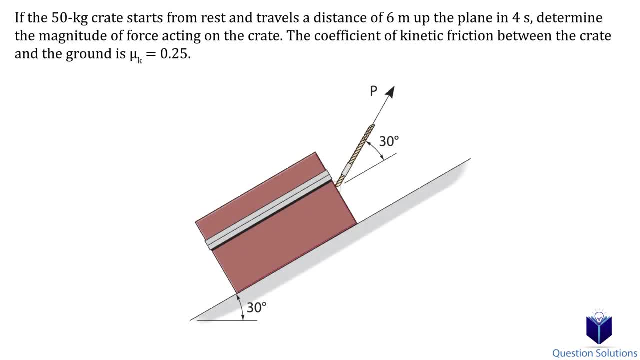 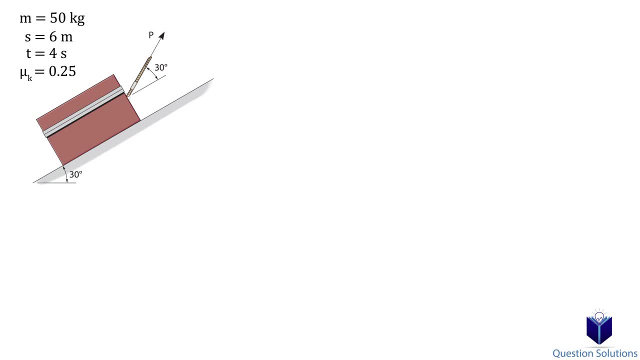 Let's look at another problem In this question. we need to figure out the force applied at the rope for the crate to move a distance of 6 meters in 4 seconds. We can start off by drawing a free body diagram. So we have force p, the weight which is always straight down the normal force. 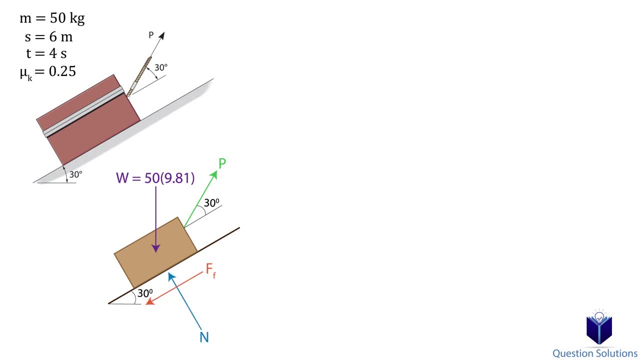 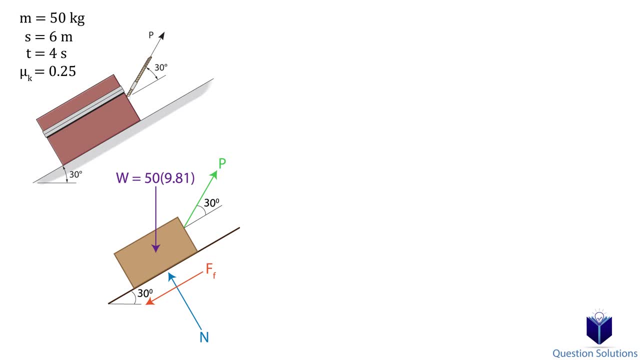 the crate moves. From the given information, we can figure out the acceleration. We just need to use a kinematics equation. Using this equation, let's plug in what we know. The final distance is 6 meters, the initial distance is 0 meters, initial velocity is 0 meters per second and the 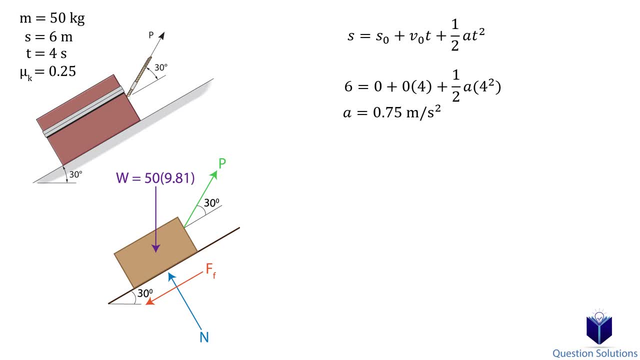 time is 4 seconds. Solving gives us the acceleration. Now we can write our equations of motion. In cases where things are on inclined planes, it's usually a good idea to pick the positive side, to be in the direction the object moves. So in this case, if our crate is moving in, 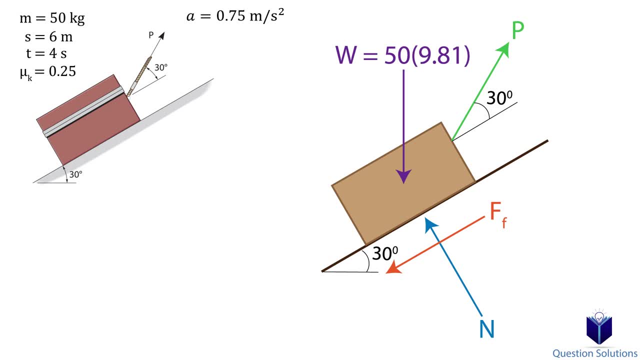 this direction, and it's on an incline of 30 degrees. that's going to be our positive direction. This makes the math a bit simpler. Another way of thinking about it is that we're placing the x-axis along the inclined plane, so the y-axis would be perpendicular to the inclined plane. 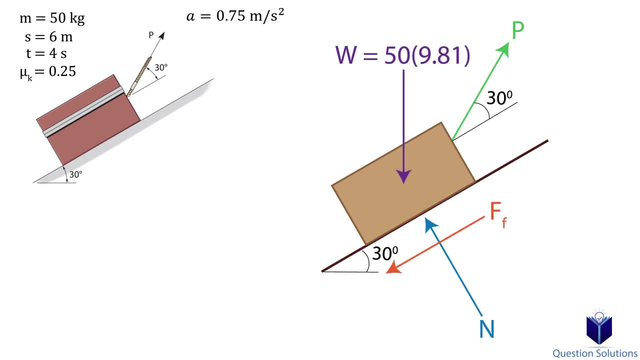 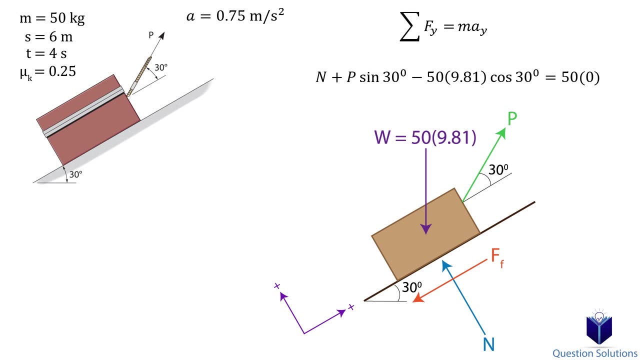 Our first equation of motion will be for the y-axis forces or vertical forces. Again, since we placed the coordinate system on the inclined plane, we don't need to break the normal force into components. So we have the normal force, the y-component of force p, the y-component of gravity. 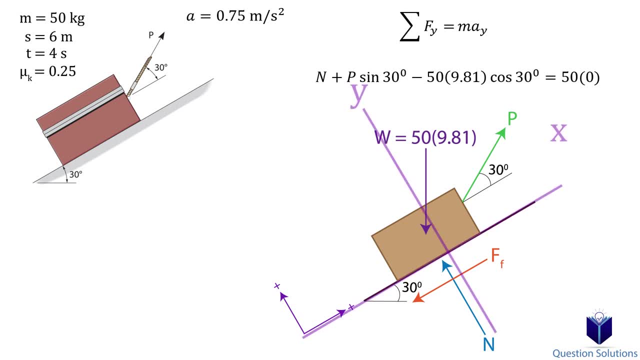 and all of this added together is equal to the mass times acceleration. But the box is only moving along the x-axis, not the y-axis, So the acceleration in the y-direction is 0.. This is why placing the coordinate system along the plane is helpful. Let's isolate for the normal force. 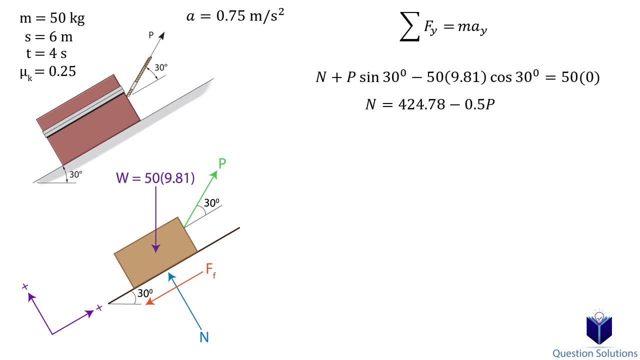 and move on to the next equation of motion. So we have the x-component of force, p, the frictional force multiplied by the normal force, the x-component of weight, and all of this added together is equal to the mass times acceleration we found earlier. We can plug in the n-value we found from the previous equation and solve for p. 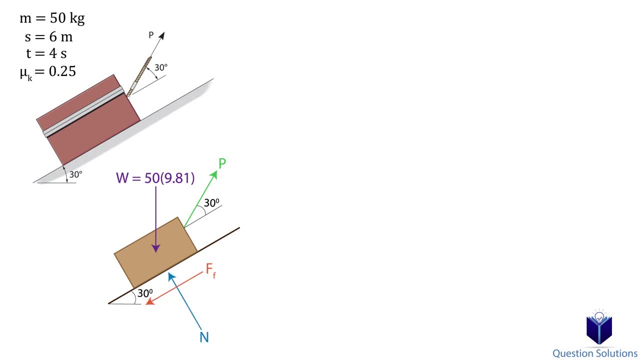 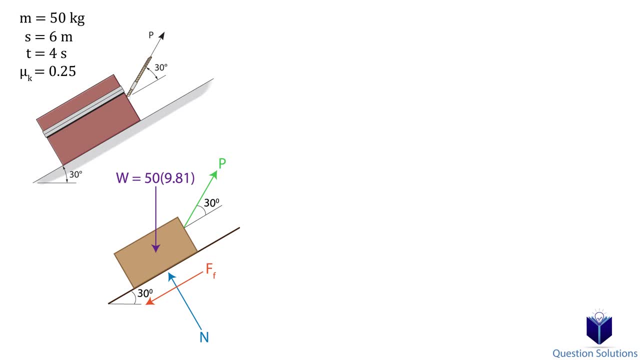 the crate moves. From the given information, we can figure out the acceleration. We just need to use a kinematics equation. Using this equation, let's plug in what we know. The final distance is 6 meters, the initial distance is 0 meters, initial velocity is 0 meters per second and the 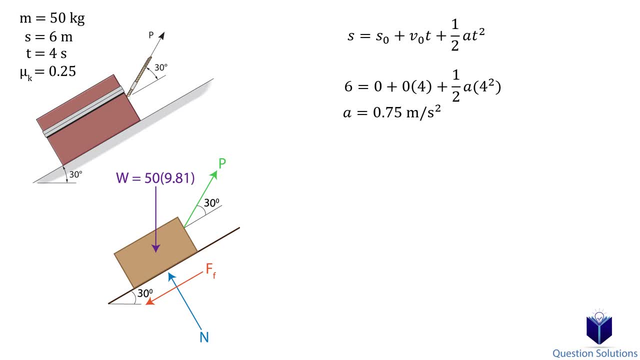 time is 4 seconds. Solving gives us the acceleration. Now we can write our equations of motion. In cases where things are on inclined planes, it's usually a good idea to pick the positive side, to be in the direction the object moves. So in this case, if our crate is moving in, 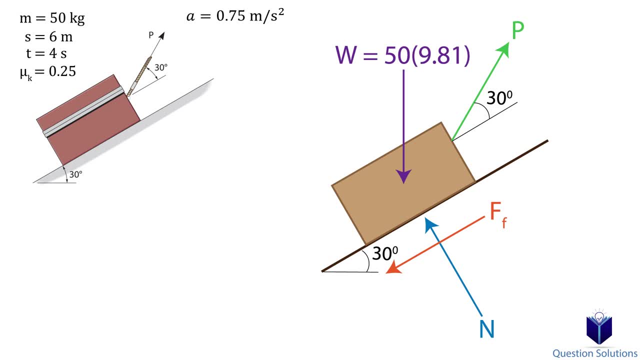 this direction, and it's on an incline of 30 degrees. that's going to be our positive direction. This makes the math a bit simpler. Another way of thinking about it is that we're placing the x-axis along the inclined plane, so the y-axis would be perpendicular to the inclined plane. 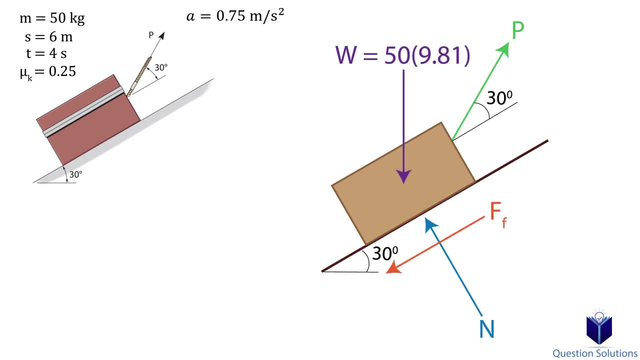 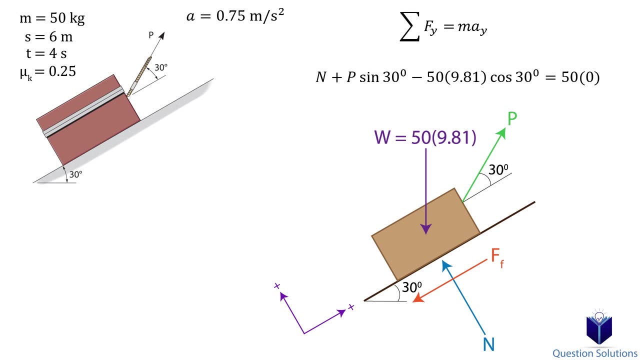 Our first equation of motion will be for the y-axis forces or vertical forces. Again, since we placed the coordinate system on the inclined plane, we don't need to break the normal force into components. So we have the normal force, the y-component of force p, the y-component of gravity. 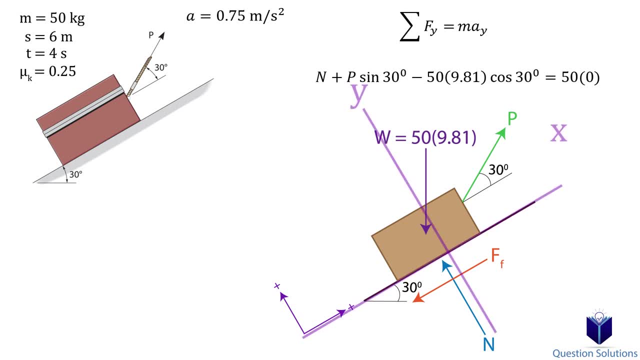 and all of this added together is equal to the mass times acceleration. But the box is only moving along the x-axis, not the y-axis, So the acceleration in the y-direction is 0.. This is why placing the coordinate system along the plane is helpful. Let's isolate for the normal force. 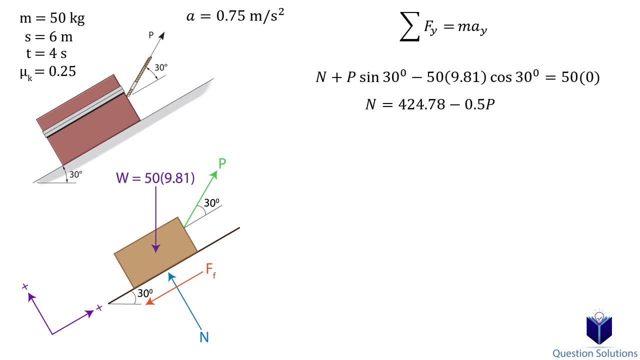 and move on to the next equation of motion. So we have the x-component of force, p, the frictional force multiplied by the normal force, the x-component of weight, and all of this added together is equal to the mass times acceleration we found earlier. We can plug in the n-value we found from the previous equation and solve for p. 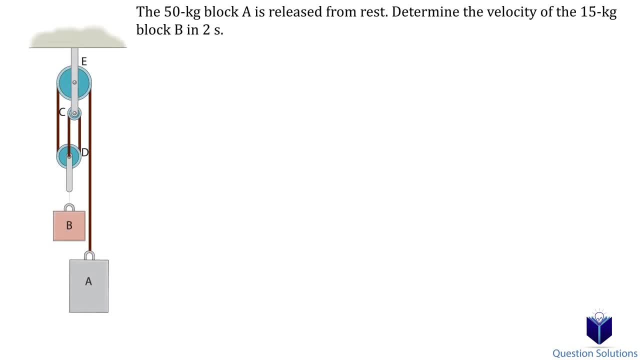 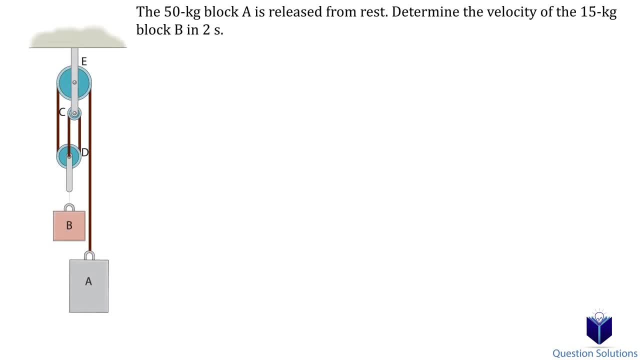 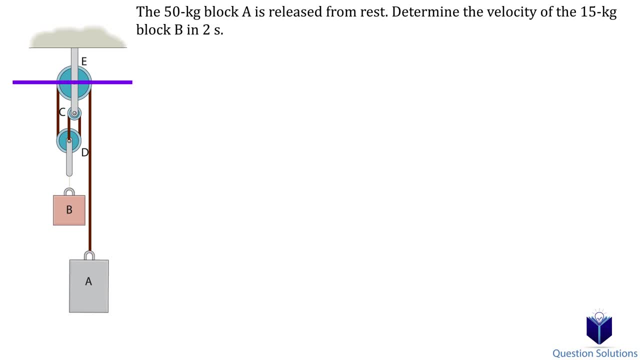 the first step is to draw a datum. We will establish it at the top pulley. We can draw two position coordinates- SA and SB- and the fixed length which we will label A. If you aren't too familiar with this, please see the description on how to solve pulley problems, The whole system. 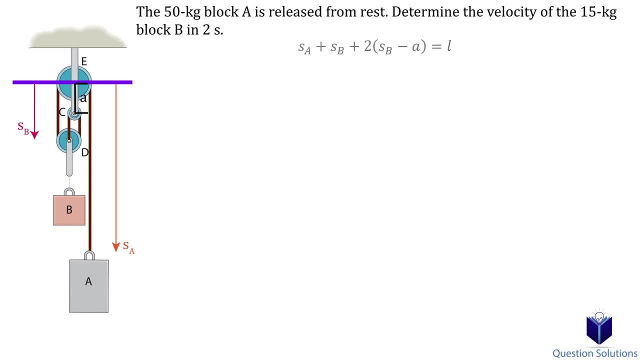 has one cable, so we only need one equation. We have SA plus SB plus 2 times SB minus A, which is equal to the total length. Let's simplify it: Taking the first time derivative gives us the velocity and taking the second time derivative gives us the acceleration. Now that we have an equation. 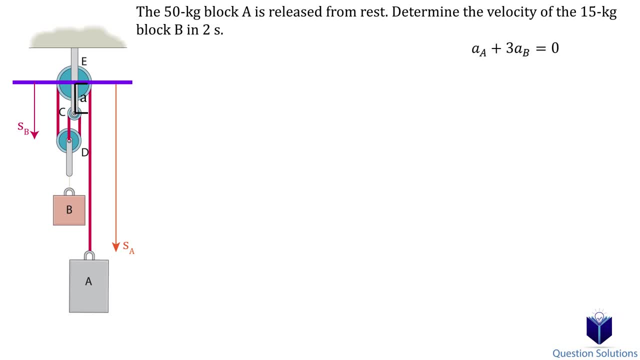 to represent the accelerations of block A and B, let's draw two free body diagrams for each of them. For block A, we only have one cable with the weight downwards. For block B, we have three cables along with the weight. It's important to note that our position 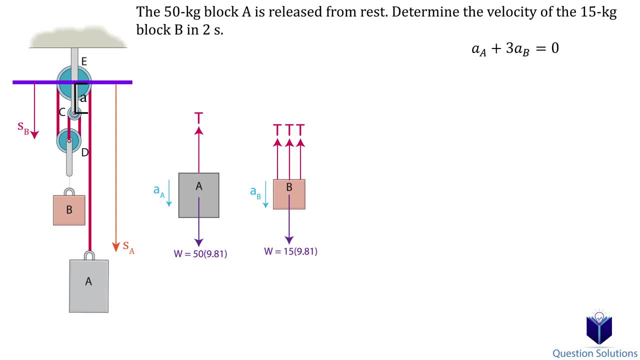 coordinates for each block was drawn downwards, meaning we picked movement downwards to be positive. So when we found the accelerations, we also assumed they're downwards as well. Now we can start writing our equations of motion. We will start with block A. 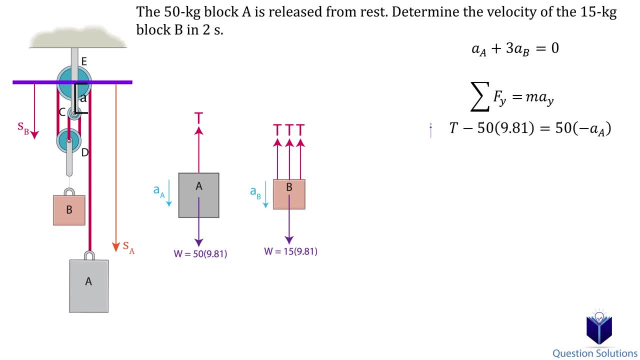 and we will write it for vertical forces. We will assume forces upwards to be positive. So we have the tension in the cable minus the weight, and all of that added together is equal to the mass times. acceleration Again, since we chose acceleration to be downwards. 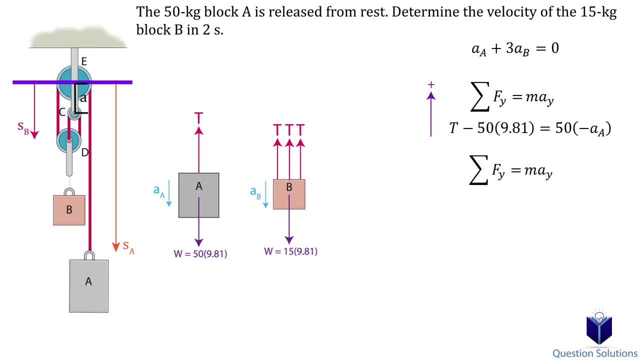 it's going to be negative. Next we will do the same for block B. We have three cables, so it's 3t minus the weight, which is equal to the mass times the acceleration. We now have three equations with three unknowns You can solve. 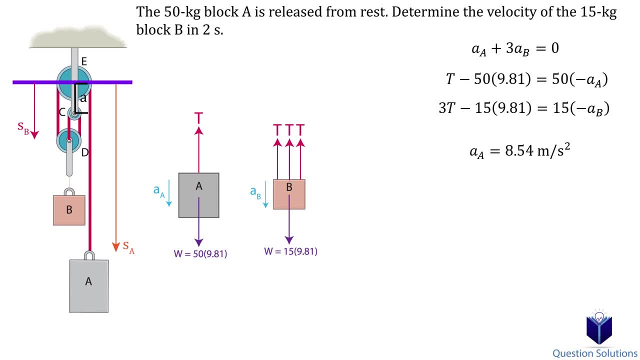 them any way you like. Solving gives us the acceleration of block A, block B and the tension in the cable. The acceleration of B is negative, which means it's actually going opposite to the way we picked to be positive. In other words, the acceleration of block B is actually upwards. 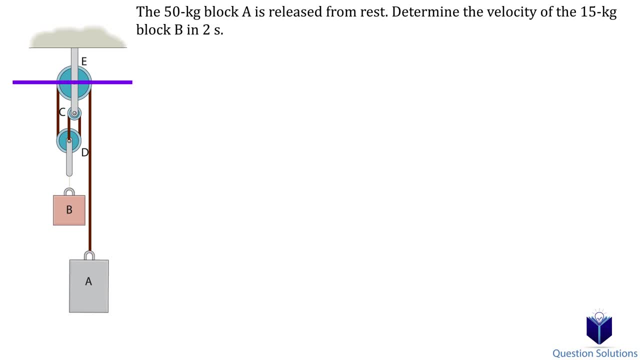 the first step is to draw a datum. We will establish it at the top pulley. We can draw two position coordinates- SA and SB- and the fixed length which we will label A. If you aren't too familiar with this, please see the description on how to solve pulley problems, The whole system. 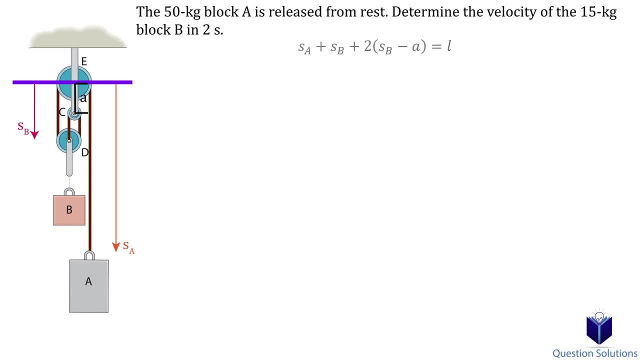 has one cable, so we only need one equation. We have SA plus SB plus 2 times SB minus A, which is equal to the total length. Let's simplify it: Taking the first time derivative gives us the velocity and taking the second time derivative gives us the acceleration. Now that we have an equation. 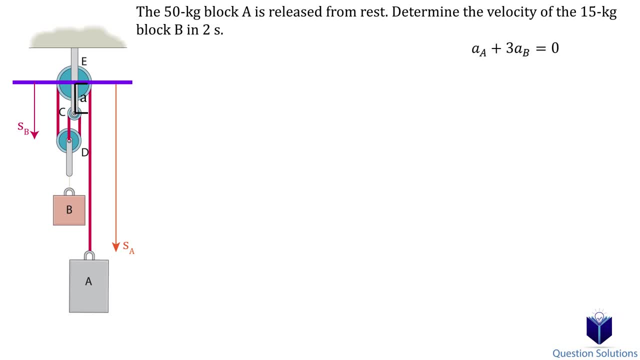 to represent the accelerations of block A and B, let's draw two free body diagrams for each of them. For block A, we only have one cable with the weight downwards. For block B, we have three cables along with the weight. It's important to note that our position 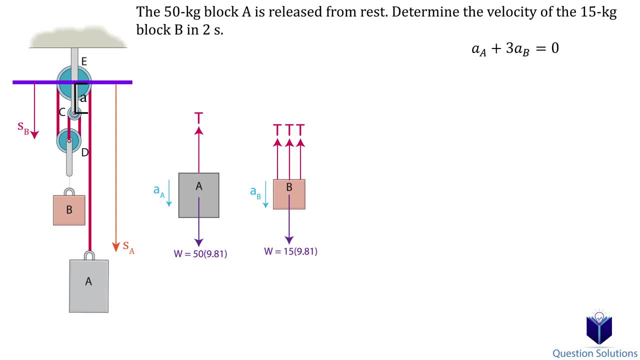 coordinates for each block was drawn downwards, meaning we picked movement downwards to be positive. So when we found the accelerations, we also assumed they're downwards as well. Now we can start writing our equations of motion. We will start with block A. 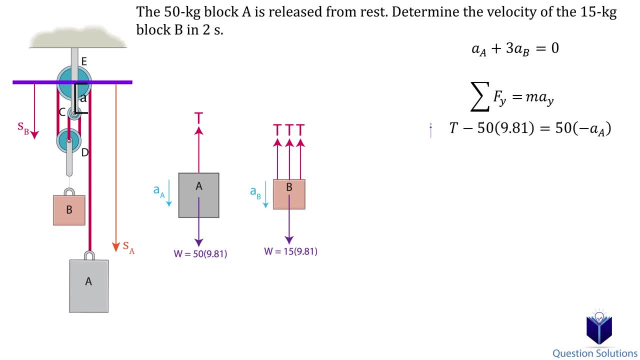 and we will write it for vertical forces. We will assume forces upwards to be positive. So we have the tension in the cable minus the weight, and all of that added together is equal to the mass times. acceleration Again, since we chose acceleration to be downwards. 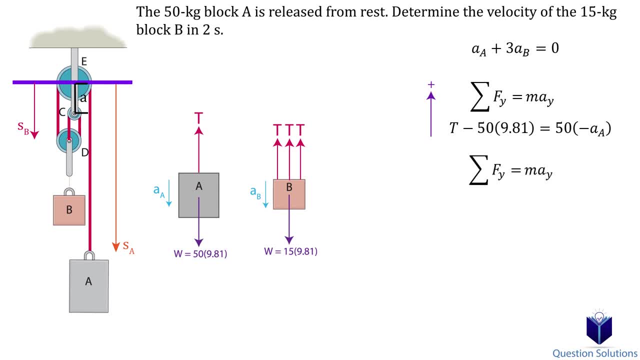 it's going to be negative. Next, we will do the same for block B. We have three cables, so it's 3t minus the weight, which is equal to the mass times the acceleration. We now have three equations with three unknowns. You can solve them any way you like. 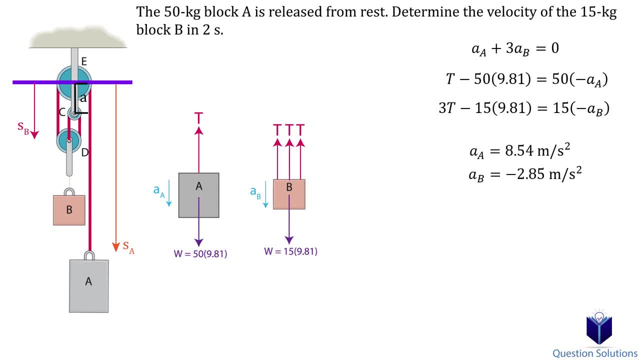 Solving gives us the acceleration of block A, block B and the tension in the cable. The acceleration of B is negative, which means it's actually going opposite to the way we picked to be positive. In other words, the acceleration of block B is actually upwards. 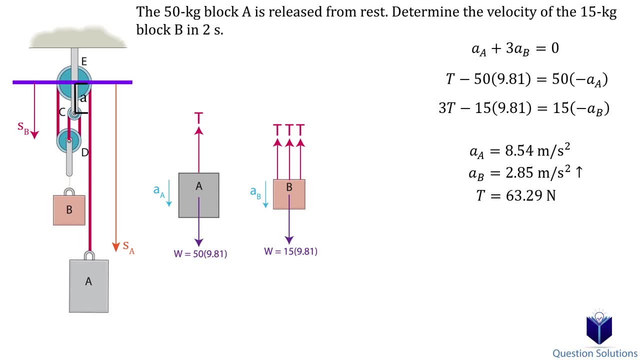 We aren't done yet. The question is asking for the velocity of block B at 2 seconds. For that we will use a kinematics equation. Using this equation, assuming up to be positive, we can start plugging in values. Remember. 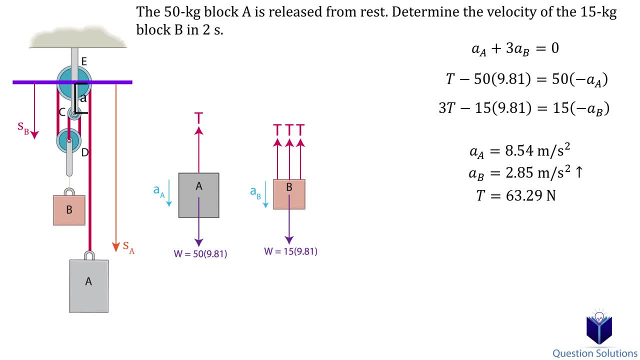 We aren't done yet. The question is asking for the velocity of the block B at 2 seconds. For that we will use a kinematics equation. Using this equation, assuming up to be positive, we can start plugging in values. Remember, this is for block B. 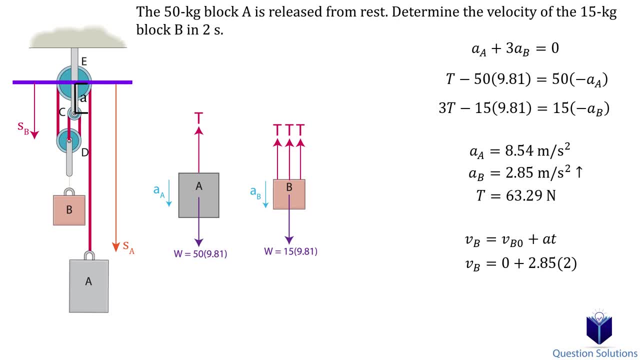 We know block A starts from rest, so that means the whole pulley system starts from rest and the initial velocity of block B is therefore 0 meters per second. We found the acceleration and the time is 2 seconds. Solving gives us the velocity of block B in 2 seconds. 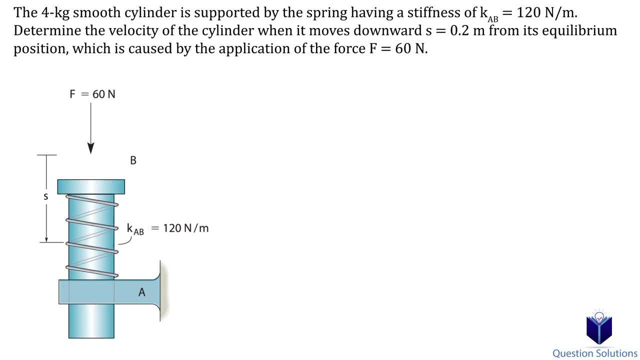 Let's look at one last example. In this question we need to find the velocity of this cylinder when it moves down 0.2 meters. So this question involves a spring, And the first thing that should come to mind is that the force needed to compress or extend the spring. 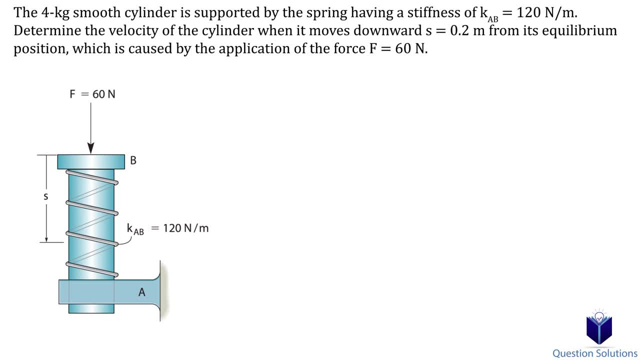 is equal to the stiffness multiplied by the displacement of the spring from its equilibrium position, also known as Hooke's law, or F equals kx. Let's first find the displacement of the spring with just the weight of the cylinder, the 60N force being applied. So we're trying to find how much the spring compresses with just the 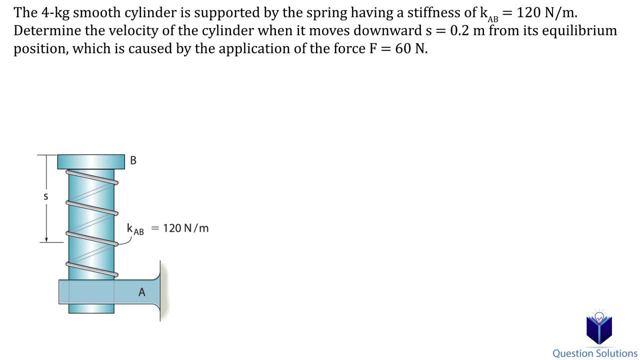 weight of the cylinder without any external forces being applied, when it's just resting. For that we can write an equation of equilibrium for the vertical forces. So we have the force of the spring minus the weight, which is equal to zero. We can solve. 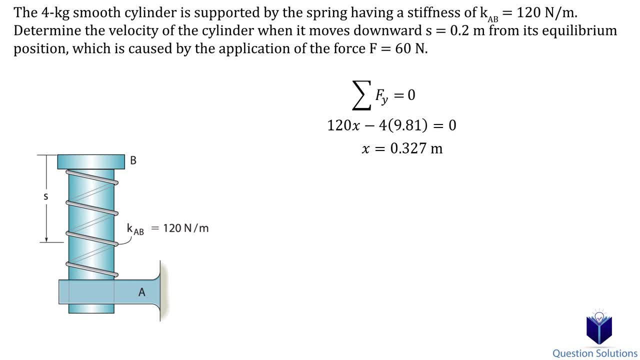 for the displacement. This value we found represents the displacement of the spring with just the weight of the cylinder. Now, when we apply another 60N of force, the total displacement is S plus 0.327 meters. Knowing this, the force of the spring is then the stiffness of the spring multiplied by S plus 0.327 meters. 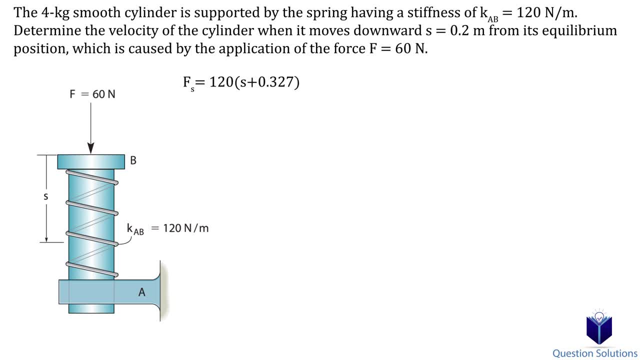 That is the total force of the spring. Let's draw a free body diagram to illustrate this. The spring wants to come back to equilibrium, so it exerts the force upwards, and that force is the stiffness of the spring multiplied by the total displacement. Let's write an equation of motion for the vertical forces and we will assume upwards. 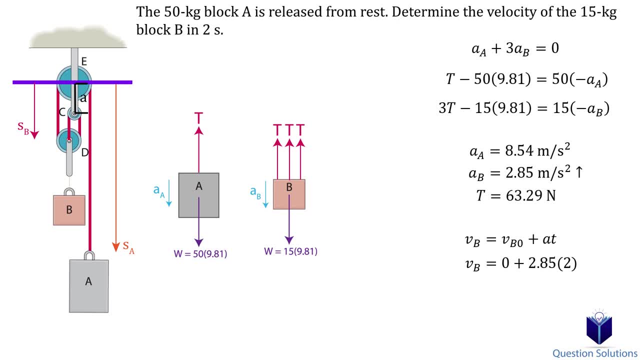 this is for block B. We know block A starts from rest, so that means the whole pulley system starts from rest and the initial velocity of block B is therefore 0 meters per second. We found the acceleration and the time is 2 seconds. Solving gives us the velocity of block B in 2 seconds. 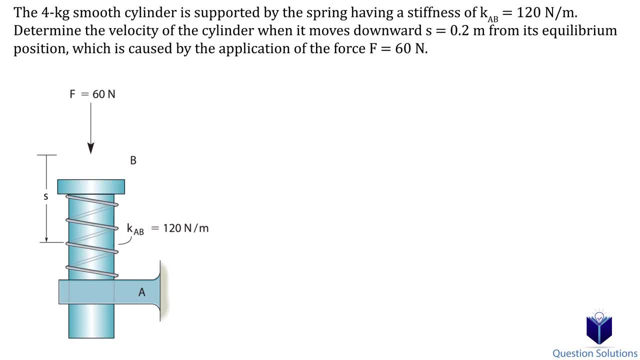 Let's look at one last example. In this question we need to find the velocity of the cylinder when it moves down 0.2 meters. This question involves a spring. The first thing that comes to mind is that the force needed to compress or extend the spring is equal to the stiffness multiplied. 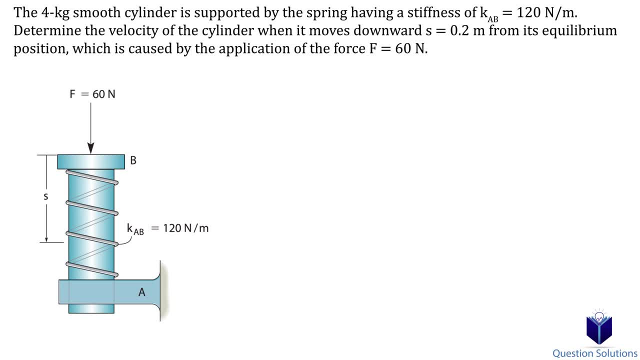 by the displacement of the spring from its equilibrium position, also known as Hooke's Law, or F equals kx. Let's first find the displacement of the spring with just the weight of the cylinder, ignoring the 60N force being applied. So we're trying to find how much the spring compresses. 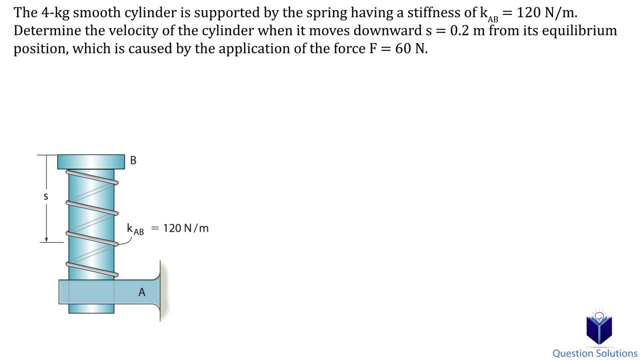 with just the weight of the cylinder, without any external forces being applied, when it's just resting. For that we can write an equation of equilibrium for the vertical forces. So we have the force of the spring minus the weight, which is equal to zero. We can solve. 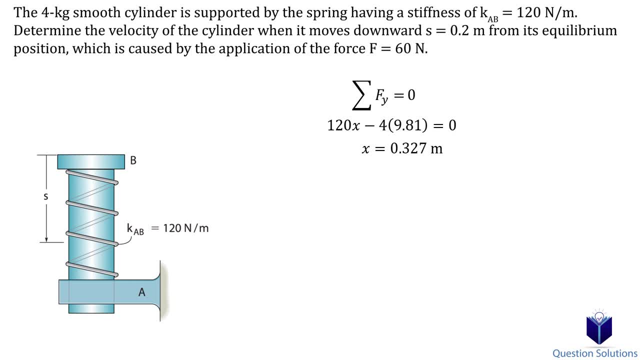 for the displacement. This value we found represents the displacement of the spring with just the weight of the cylinder. Now, when we apply another 60N of force, the total displacement is S plus 0.327 meters. Knowing this, the force of the spring is then: 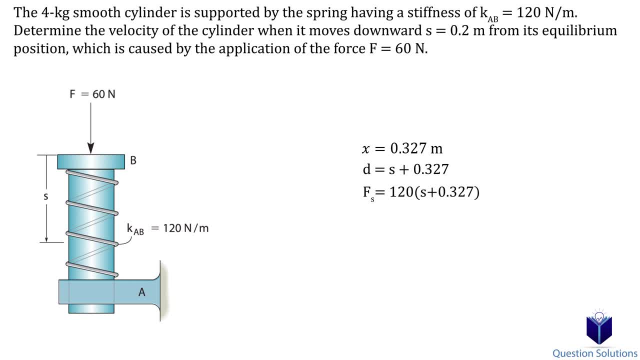 the stiffness of the spring multiplied by S plus 0.327 meters, That is the total force of the spring. Let's draw a free body diagram to illustrate this. The spring wants to come back to equilibrium, so it exerts the force upwards, and that force is the stiffness of the spring multiplied by the. 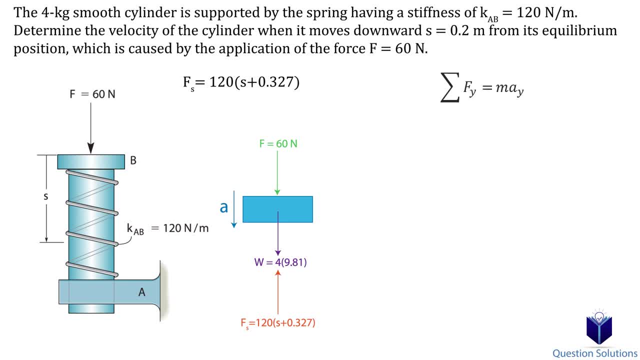 total force of the spring. This is the difference between the force of the spring and the weight of the cylinder displacement. Let's write an equation of motion for the vertical forces and we will assume upwards to be positive. So we have the force of the spring, the force applied from top, the weight. 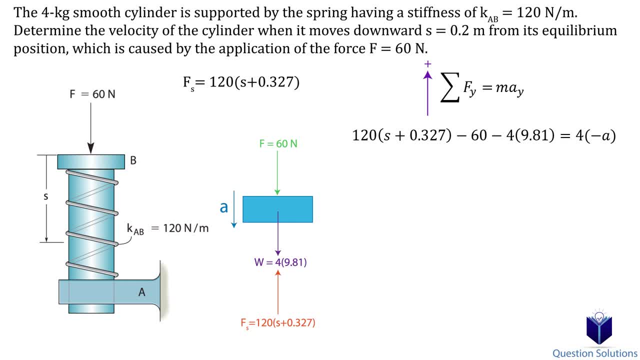 and all of this added together is equal to the mass times acceleration. Since the cylinder will move downwards, the acceleration will also be downwards, meaning it's negative a. Let's isolate the equation for acceleration. Now we have an acceleration equation with respect to displacement.